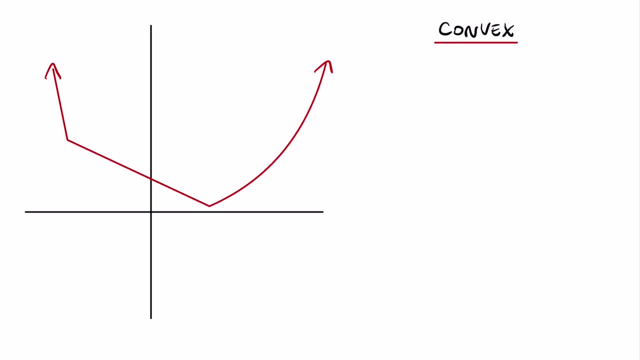 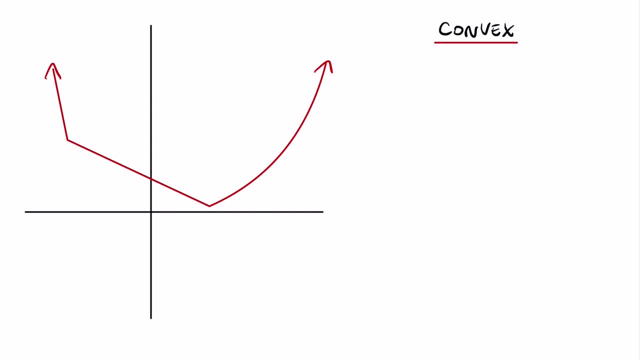 of what a convex function is, And I intentionally drew an example- that's not differentiable. We notice that we have these two points that would cause problems for differentiability, and the reason why I introduced these is so we have a concrete working definition that avoids. 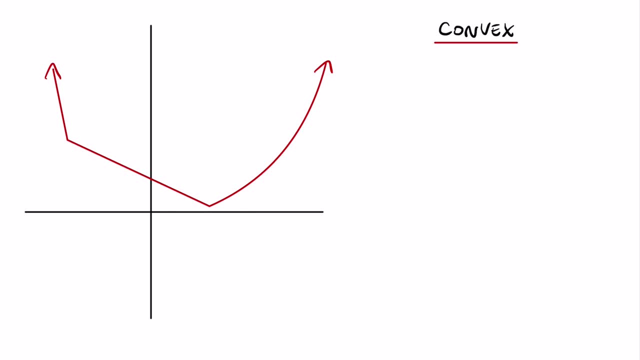 the necessity of talking about derivatives. So let's get a sense of what this ought to be. So let's say we pick two points- x and y- and look at the outputs of those points. So these points on the graph are y- f of y- and x- f of x. 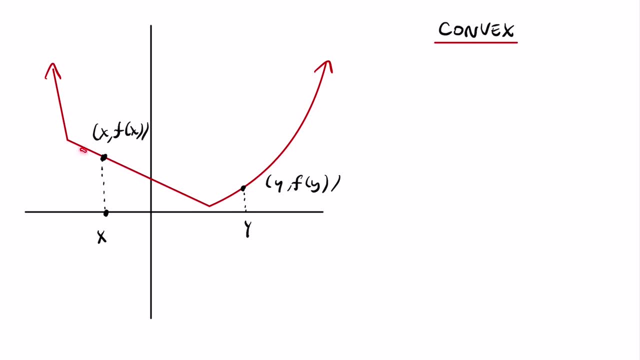 Now the whole idea about being convex is that this region above the graph never dips into something like this. You don't have these sort of like holes here. So how do we talk about that concretely? Well, we can look at the line segment between these two points. 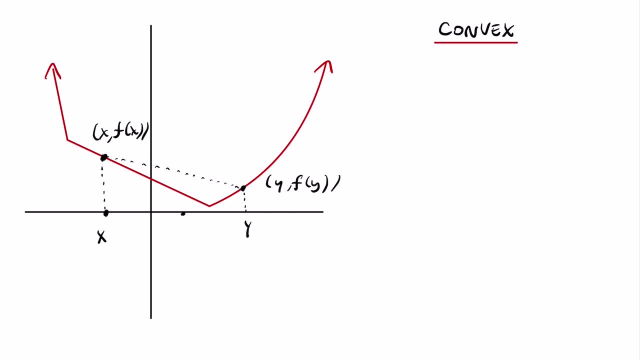 x- f of x and y- f of y. Now, if we take any intermediate point, call it z or z, then we have two things we can consider. One is the point right over here, which is the point on the graph, which is z or z- f of z. 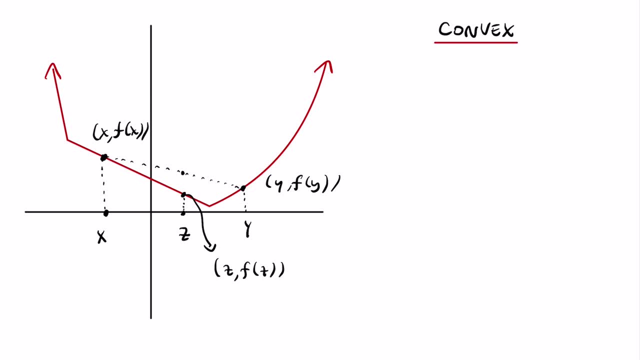 Then we have this other point, which is on the line segment between x- f of x- and y- f of y, And we need to talk about that concretely. z itself is on the line segment between x and y, So we can actually write it as t x plus 1 minus t y, where t is a value between 0 and 1.. 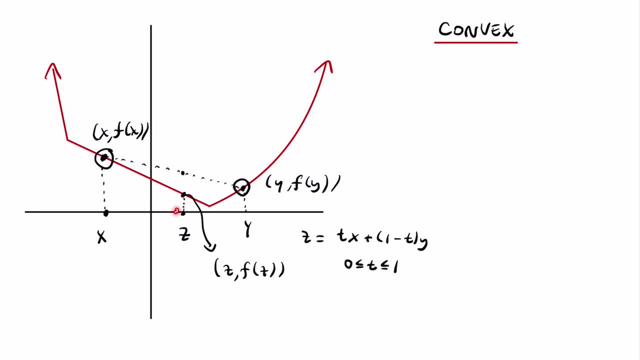 For example, if z was right at the middle of the line segment between x and y, then t would be a half, So we'd have a half x plus a half y. It would be the average of the two points. However, if it was somewhere like here, it would be like three quarters x plus a quarter y. 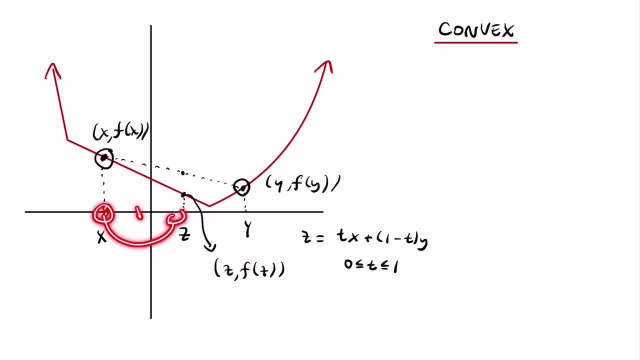 It'd be halfway through between x and the midpoint of x and y, And any general point on this line segment can be represented in this way. So that means this point on this graph is t, x plus 1, minus t, y and f at that value. 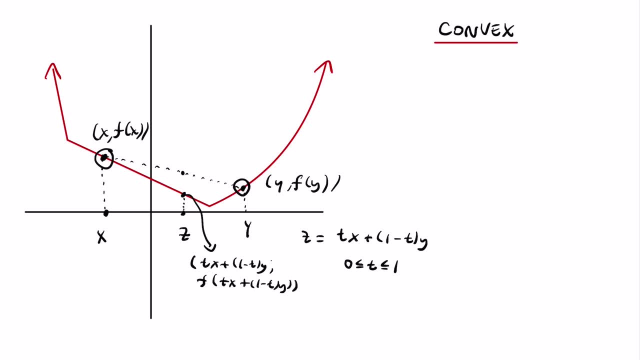 f at t x plus 1 minus t y. Okay, but what about this point right over here? If this function is convex, the geometry that we're seeing is that this point on the line segment between these two points should lie above this point right over here. The coordinates of this point, because of the scaling, are tx plus 1 minus. 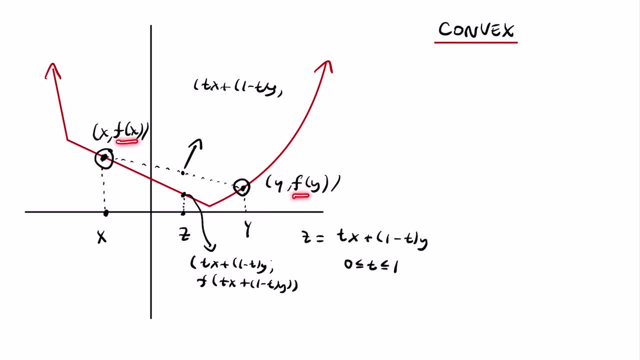 ty, and then a scaling of these two coordinates here by these t and 1 minus t values, which is t f of x plus 1 minus t f of y. Okay, so for a function to be convex, we need always that this y coordinate here is greater than or equal to this y coordinate here. So we can now 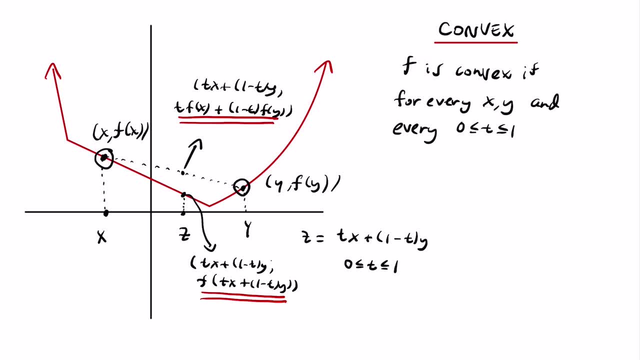 state this concretely: f is convex if, no matter what two points- x and y- you select in the real numbers and value t between 0 and 1, the function value evaluated at tx plus 1 minus ty is less than or equal to t f of x plus 1 minus t f of y. Now again to get back to this: 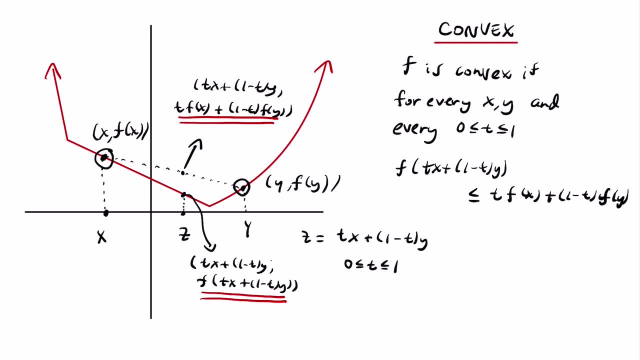 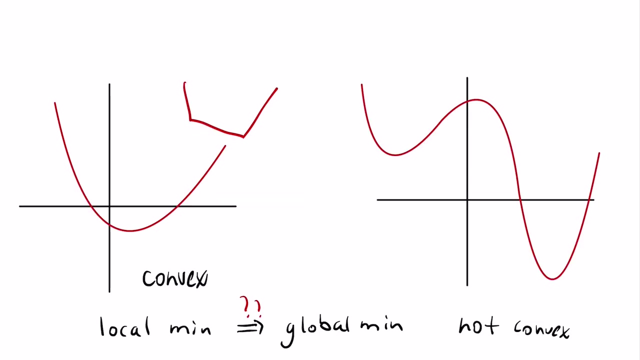 intuition of this. imagine t was a half. then we're saying here that f at a half x plus half y, meaning f, at the midpoint of these that might be here, is less than or equal to a half fx plus a half of y, which is this point right here in this y coordinate. Okay, so let's go back. 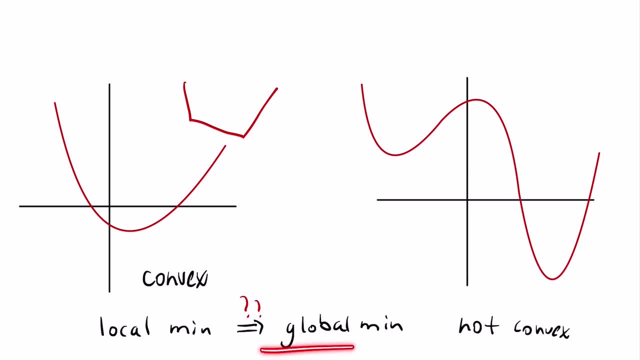 and actually see why local mins for convex functions are forced to be global mins. now that we've got a working definition of what a convex function is, Alright, we need to go back to the idea of what a local minimum is in the first place. So if you pick a point x, it's a local minimum if 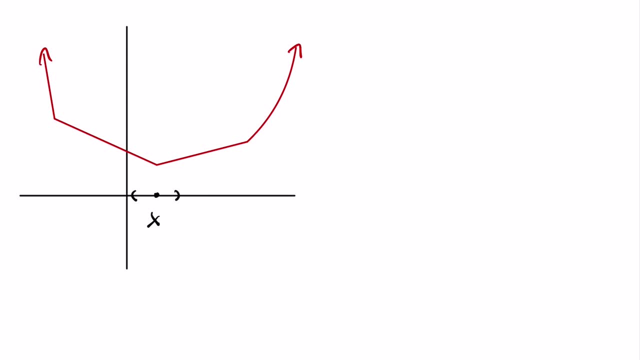 you can find a little neighborhood around it so that this function value at this point is smallest among all the points inside of this interval. Okay, so to make this special, let's call this x star and we'll say x star is a local minimum. Then we can find a small interval length. let's call it delta greater than zero. 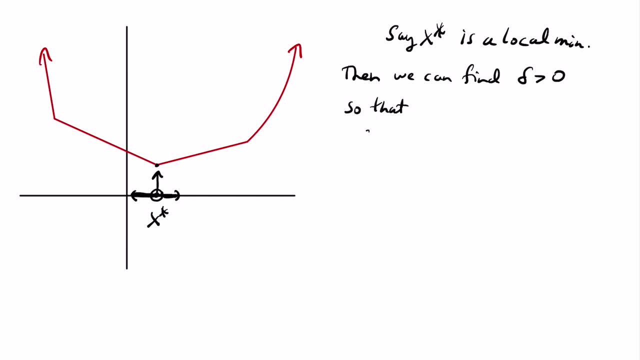 so that f of y is greater than or equal to f of x star for every y inside of this interval whose length is delta, So every y in the interval between x star minus delta and x star plus delta. So it's that small neighborhood we get that f of x star is a minimum. 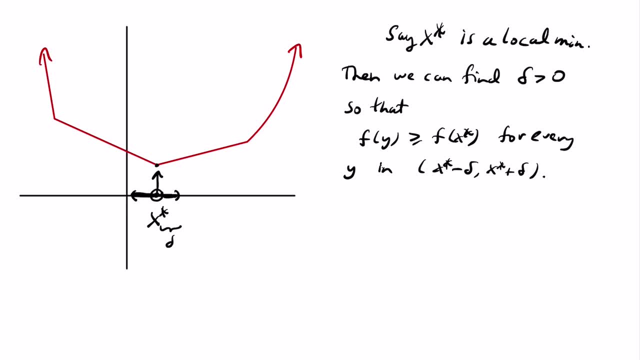 Now I want to know why x star actually is a global minimum. So say, we picked another point, z, far, far, far away. for some reason it's going to be forced to be the case that the function value at z is greater than or equal to the function value at x star. So the motivation is that 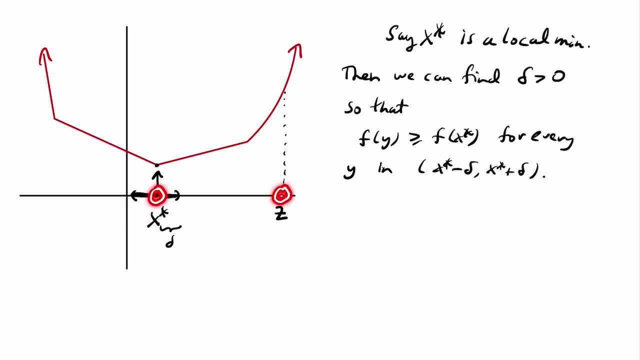 since we know something about points on the line segment between these and their function value. what we'll do is pick a point between these two values: x, star and z. that's inside of this neighborhood, and so it's going to be something whose value, when evaluated at f, is at least. 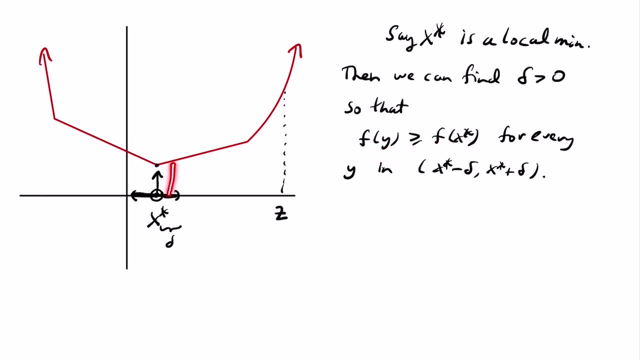 f of x star, but together with the convexity relation, we're going to be able to say something about f of z. Okay, so we'll let z be arbitrary, some real number. Then there is some value of t, and I'm going to make t strictly between zero and one, so it's not going to 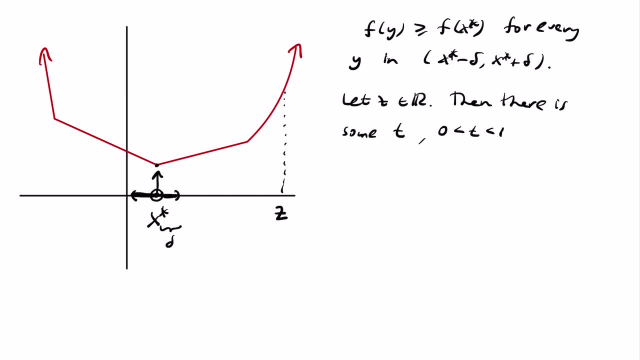 give us a point that's x star or z itself, So that x t times x star plus one minus t z is equal to f of x star. So we're going to make t strictly between zero and one. so it's not going to give us a point that's x star or z itself. 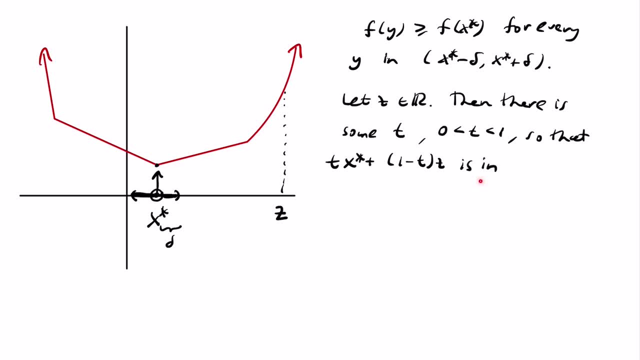 is in this interval right over here, right. the idea is: we have x star, here z, here we pick a t ever so large. so that is very, very close to x star. so it's in the interval x star minus delta, x star plus delta. Okay, so what does that mean? Well, it means that f of t, x star. 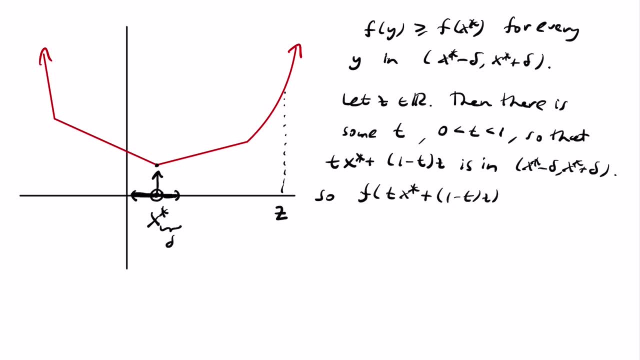 plus one minus t z. this point, that is in this interval, because x star is a local min, is going to be greater than the value of f of x star, but at the same time, because of our convexity, this value here is less than or equal to t f of x star. 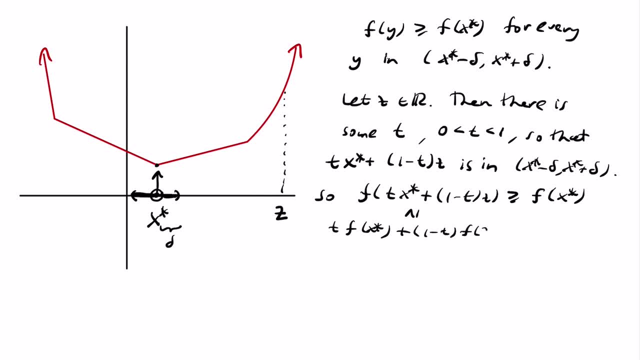 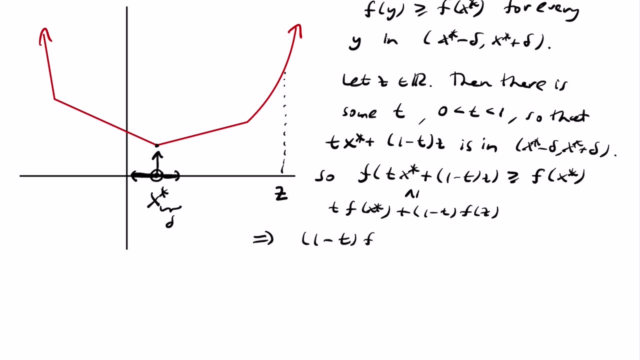 plus one minus t f of z. So we have that t f of x star plus one minus t f of z is at least f of x star, and if we rearrange that tells us one minus t f of z is at least one minus t f of x star. 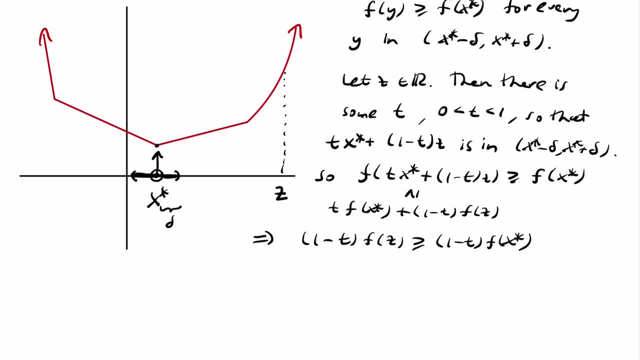 And now, because one minus t is between zero and one, because t itself was between zero and one, we can divide these two values out and get exactly the conclusion we wanted: that f of z is at least f of x star. So the motivation and idea behind this is in a. 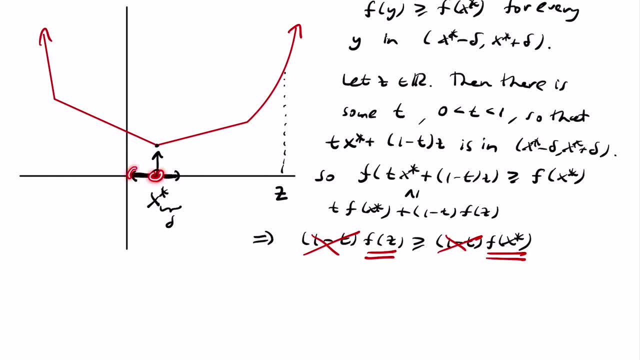 convex function. any local minimum is a minimum in a small interval. but because anytime you pick a point you can find a point on the line segment between that and x star to force it to be inside of this very small interval, convexity will allow you to establish that the function value at 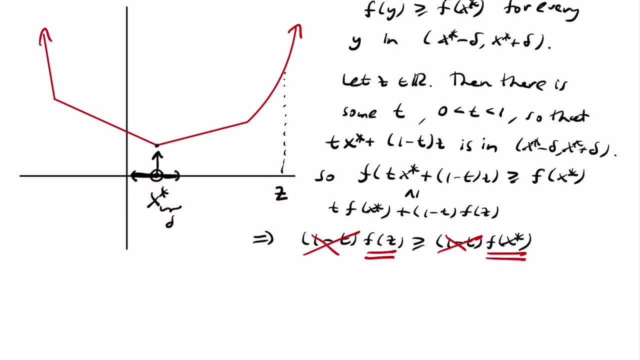 that point is actually greater than equal to the function value at that local minimum, making that local minimum actually a global minimum.